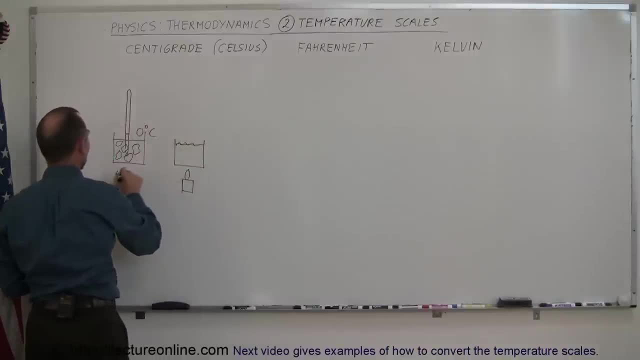 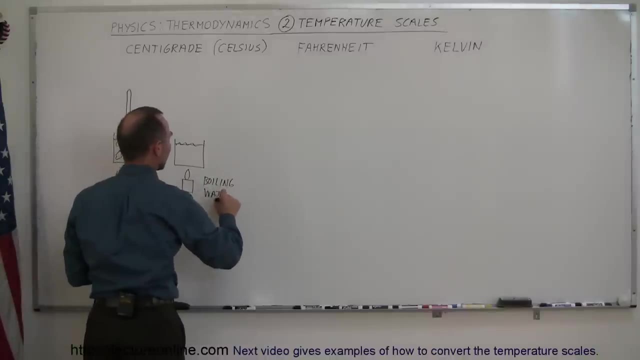 until it begins to boil. So this is a melting of ice, melting ice, and this is boiling water. And now we stick that very same temperature thermometer into the pot of boiling water, like so. Now the temperature will read 100 degrees centigrade. Of course, both of those. 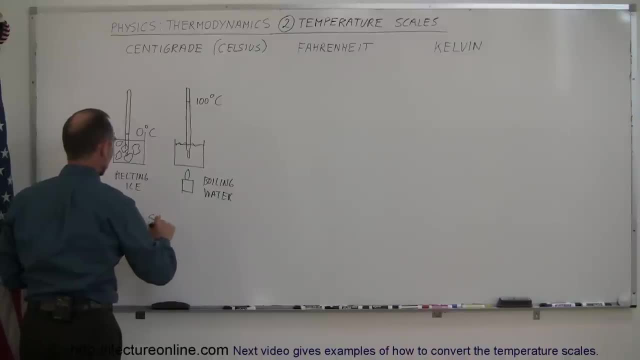 things have to occur at standard temperature. So if you take a thermometer and you put it in a consequences with water before you switch it on, like so, If you don't switch it on, the temperature is changing and then, happily, we find up to a hundred centigrade. So what will you do? 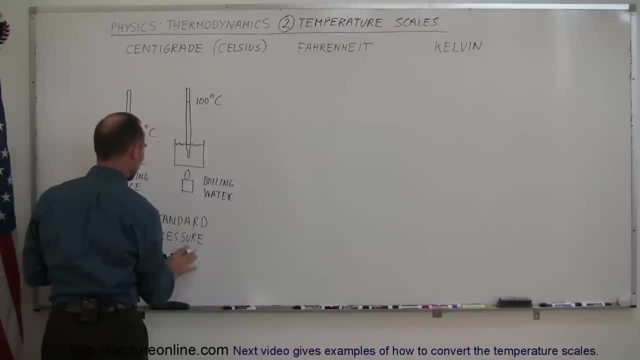 We're finding that it's going to be exactly the same temperature. How will youakov we're might call it 100 degree centigrade For what you're using currently. the temperature will be changing. Approximately we'll find Up to a hundred. 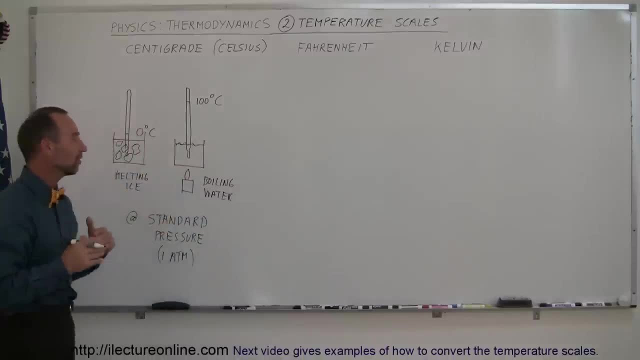 And we'll also find that a hundred centigrade high. And then, similarly, What should we do if we drink similar water, A standard pressure, Because we find that the boiling point of water will change under different pressure and also, to some extent, the 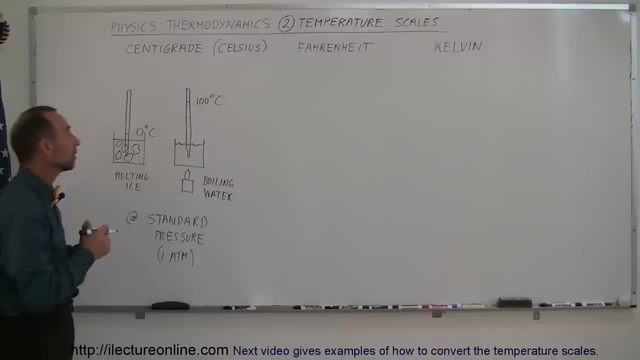 melting point of ice will also change at certain Uhp, Papa Pressure, So standard pressure, That low pressure is so exactly one atmosphere water. We'll find in then, Of course, the difference in the temperature between boiling water and melting, hundred centigrade degrees. so then we take that, that thermometer, and we divide it into 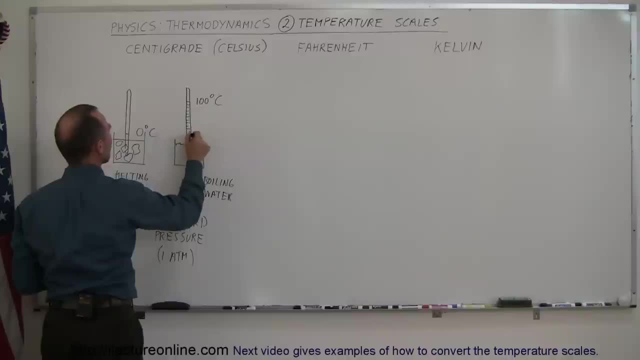 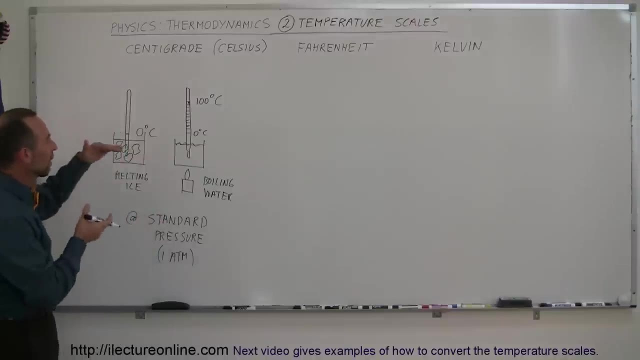 say one, two, three, four, five, six, seven, eight, nine, ten- this is the zero degree centigrade- and then we divide all of those into ten equal little lines. like that you can see that very easily. we can make a thermometer that then is scaled between zero and a hundred, representing the temperature between. 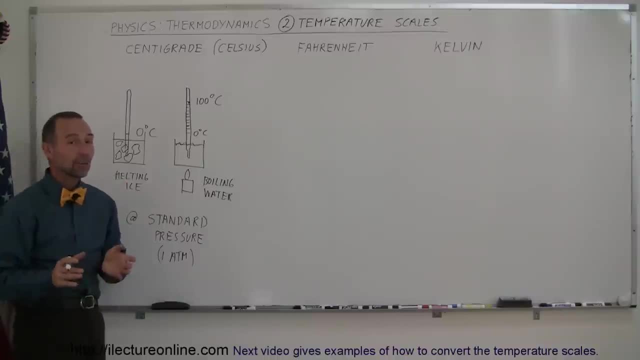 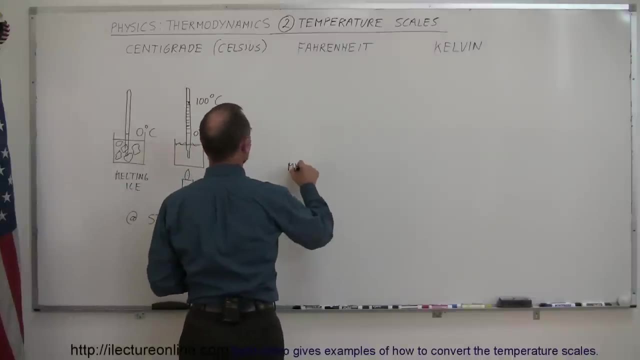 melting ice and boiling water all right now. if we do that with a thermometer that has fahrenheit degrees on it, you'll get a different result. for the case of melting ice or freezing water, the temperature- the temperature in fahrenheit degrees, so temperature in fahrenheit degrees will be equal. 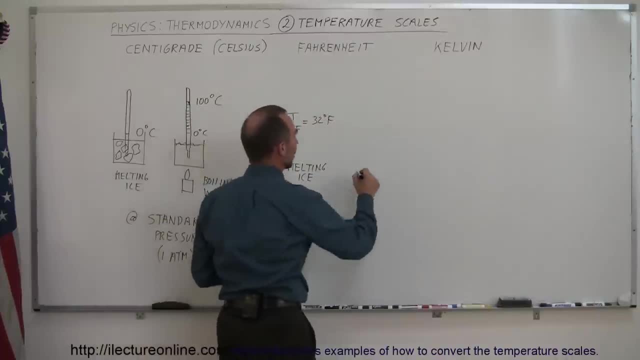 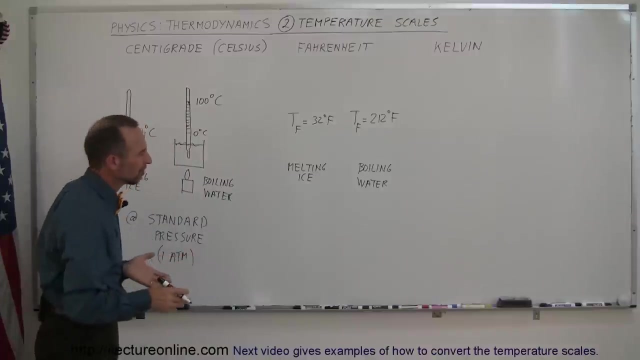 to 32 degrees fahrenheit. and if we put it in boiling water under the same circumstances- boiling water- the temperature will now read in fahrenheit degrees will be 212 degrees fahrenheit. now notice that that's quite a bit different. you say, well, that seems kind of hot. they obviously didn't use. 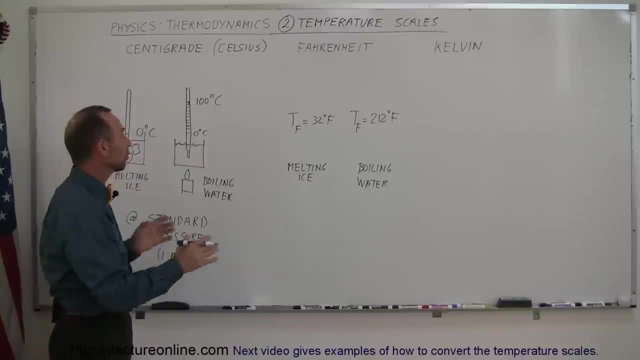 melting ice and boiling water to come up with that, that scale. but you can now see the relationship that zero degree centigrade is the same as 32- 32 degrees fahrenheit and 100 degrees centigrade is the same as 212 degrees fahrenheit, and in later video i will show you how to convert. 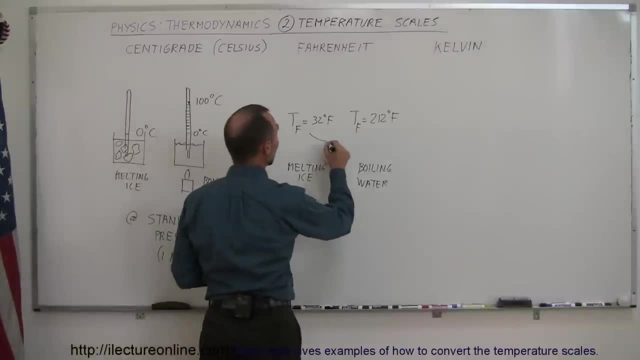 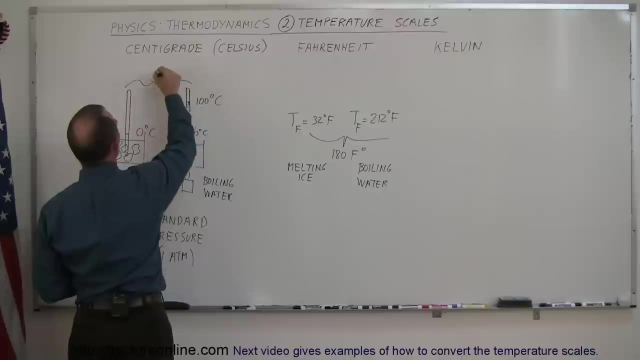 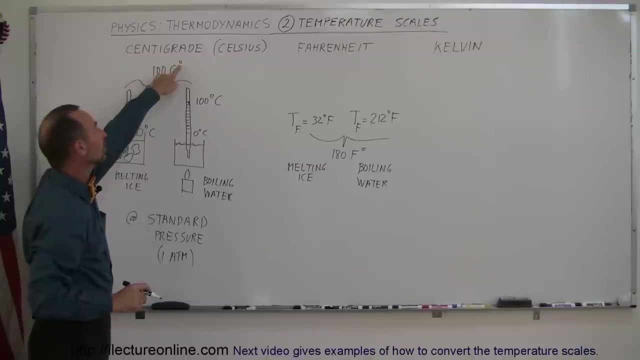 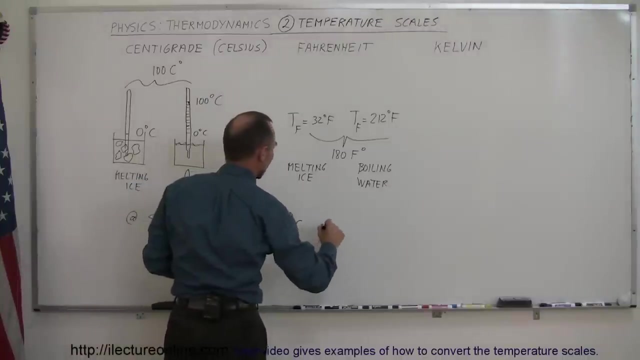 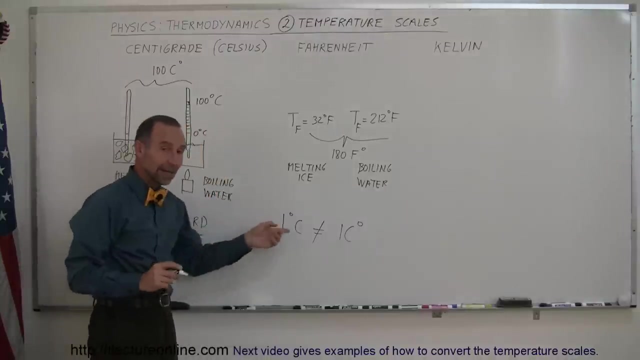 from one to the other. you just have to notice that if you take the difference between those, that is 180 fahrenheit degrees, and if you take the difference between those two, if you take the Minute degrees and two, whereby the difference between 14 and 50 degrees fahrenheit degrees- before i think for degrees- is going to be 20 degrees fahrenheit degrees, so that is 100 centigrade and body weight is 10 أ Kirkby degrees, That is 100 centigrade degrees. Now notice where i put the little symbol for degrees here. i put it behind. they're put in front. so what's the difference? what is the difference between one degree centigrade and one centigrade degree? they are not the same thing. one degree centigrade is the actual temperature. it's one degree above zero. one centigrade degree is really the difference between two. let's say the difference. 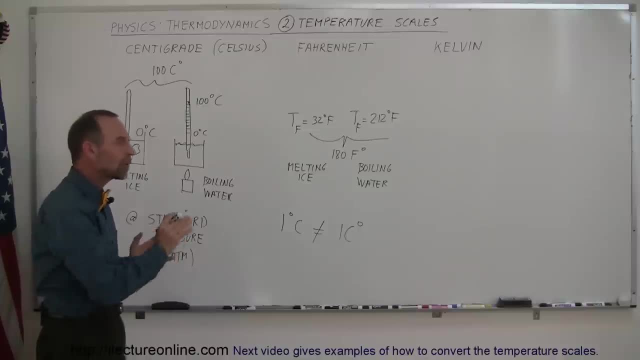 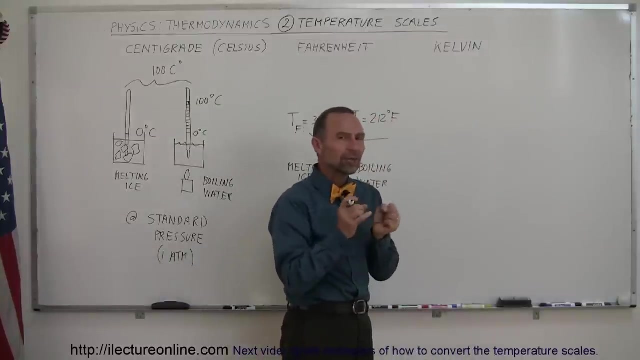 between 14 and 15, or 18 and 19 and so forth. so that's how we denote that. it's not very commonly used, but just sometimes it makes sense to keep that straight. now we have one more scale. that scale is the kelvin scale. now, the kelvin scale was formed because we recognize that there is an 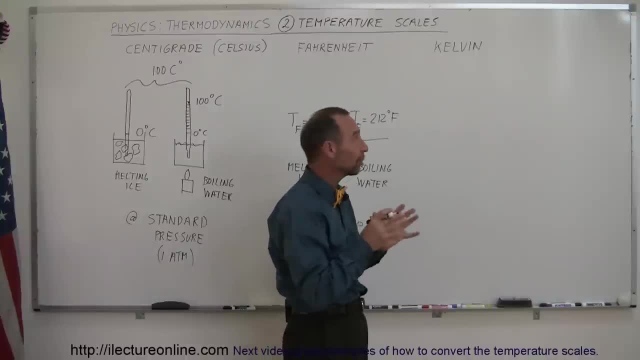 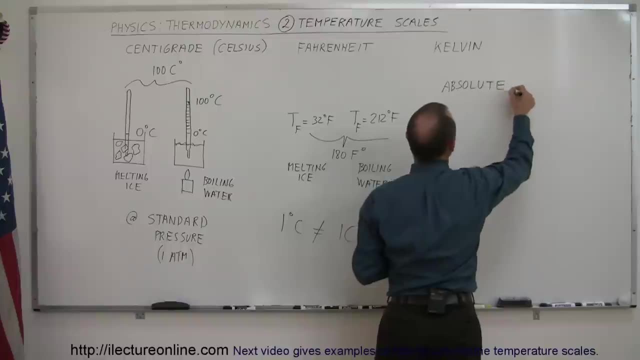 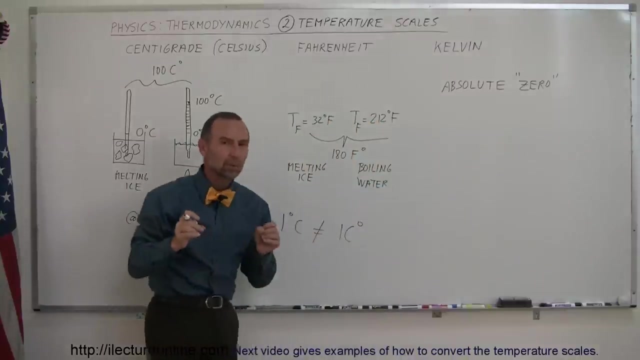 absolute temperature in the universe, the coldest it can possibly get, and that's called absolute zero. now how does something become absolute zero in temperature? absolute zero temperature? well, it turns out again. remember what heat was. heat was energy that's contained in objects, causing the atoms to vibrate back and forth. the more heat you put in the object, the hotter. 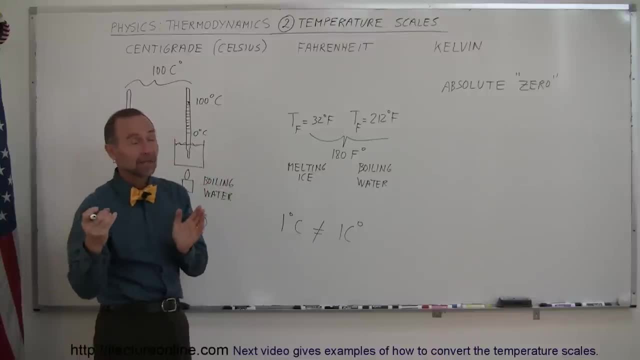 the temperature, the faster begin to vibrate. the more heat you take out of the object, the lower the temperature, the lower the atom, or the, the less the atoms will vibrate and if we continue to cool down enough and no more heat, we're not going to get the ejection of a gas. 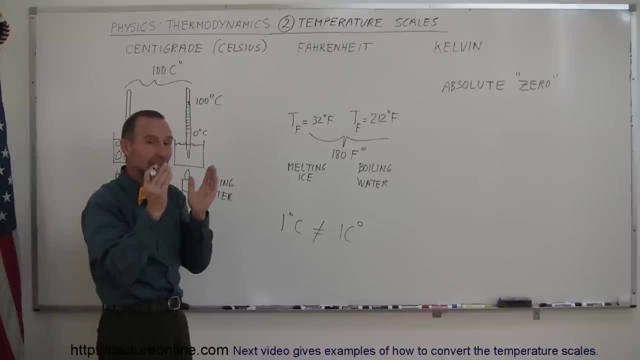 object. by taking out more and more heat out of the object, we can actually get the molecules in the atoms of the object to vibrate so slow that eventually they will essentially stop moving. The only movement they have then is quantum mechanical movement, and we're not going to. 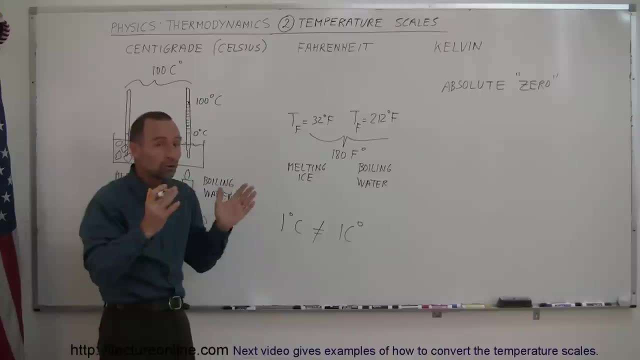 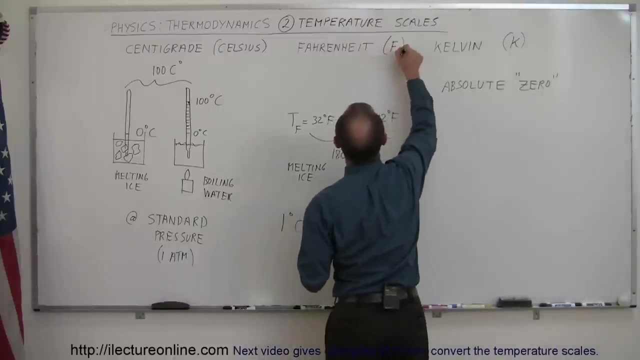 get into that detail. For our purpose, we can simply say: when all motion in the object stops, that object will be as cold as it can possibly get. That's absolute zero. Now, what is that? What is that? So, in Kelvin degrees, we use the symbol K. In Fahrenheit degrees, we use the symbol. 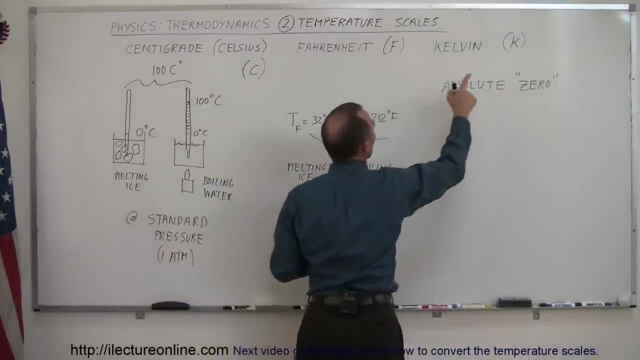 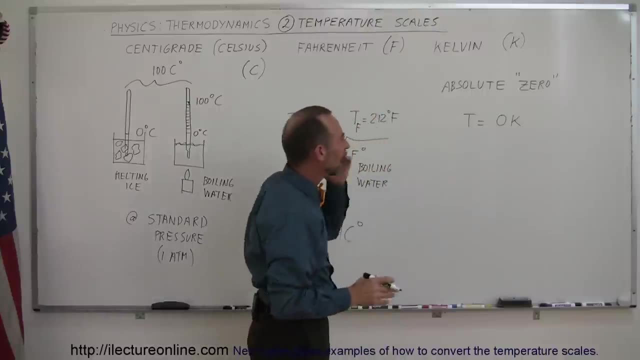 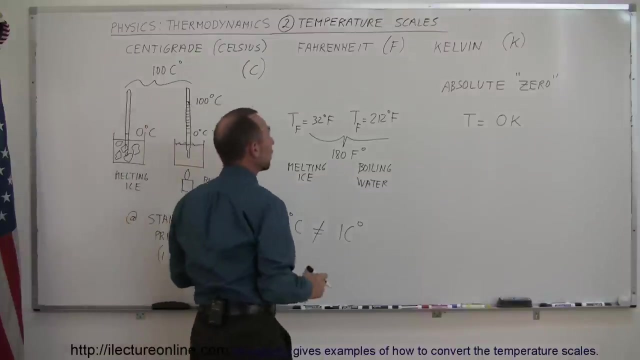 F, And in Celsius degrees we use the symbol C, And so for absolute zero, the temperature then is equal to zero Kelvin. Now we sometimes- yeah, we- don't put a degree symbol on Kelvin, by the way. so just simply zero Kelvin, And if we equate that to centigrade degrees, that is equal to minus. 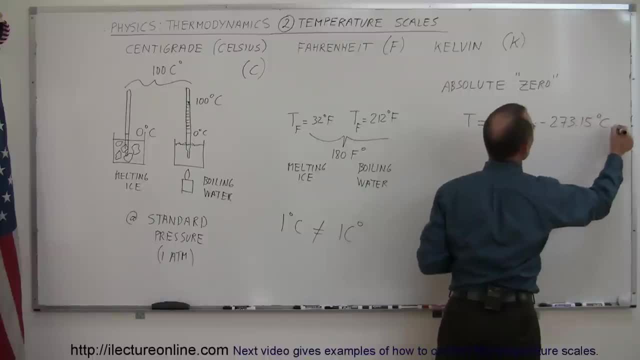 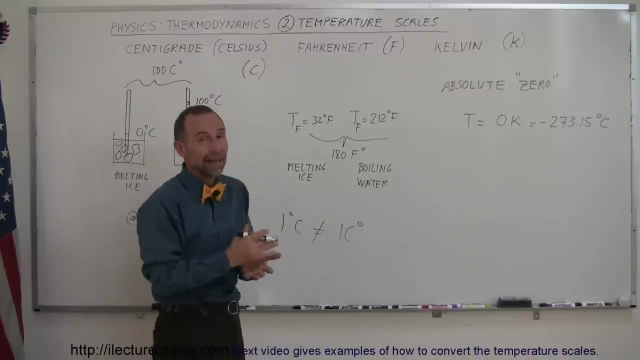 273.15 degrees centigrade. Now, the .15 is not really necessary, just to be a little bit more exact. Most of the time we simply say: zero Kelvin is equal to minus 273 centigrade degrees, or degrees centigrade. 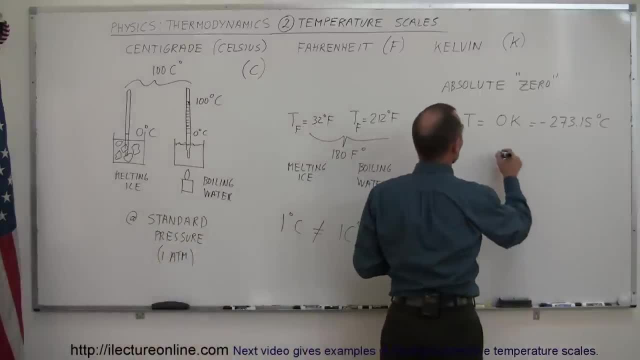 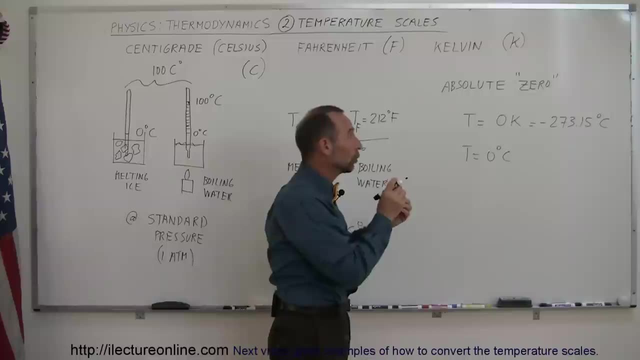 All right, so that means that zero centigrade. so if the temperature is equal to zero degrees centigrade, which is 270 degrees warmer than that- and, by the way, a degree centigrade is the same as a degree Kelvin- they're the same size. so you can see that these are not the same size. 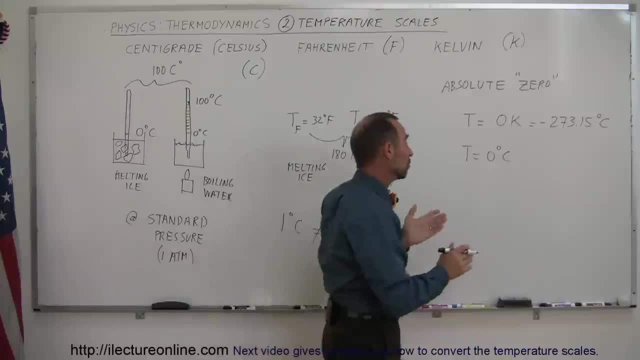 but Kelvin degrees and centigrade degrees are the same size, which means that when the temperature is zero degrees centigrade, that is equal to 273 Kelvin left off the .15.. So there you can see the comparison. And then 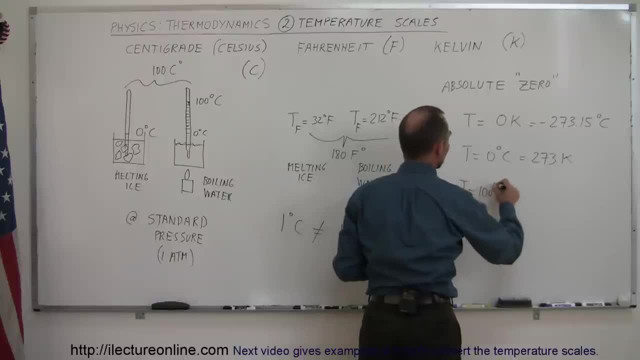 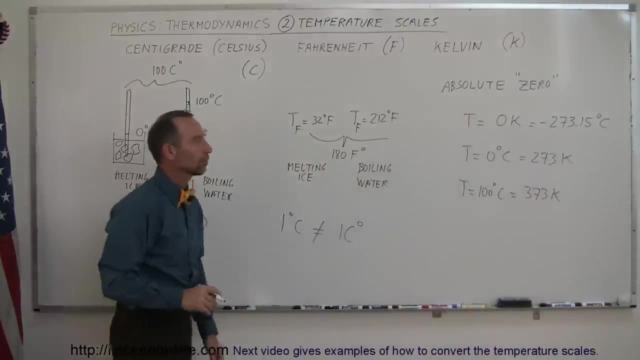 of course, if the temperature is equal to the temperature of boiling water- 100 degrees centigrade, which means that this is 373 Kelvin- We simply add 100 to each and you can see how they compare to each other. But at least now you get some sort of idea about the three temperature. 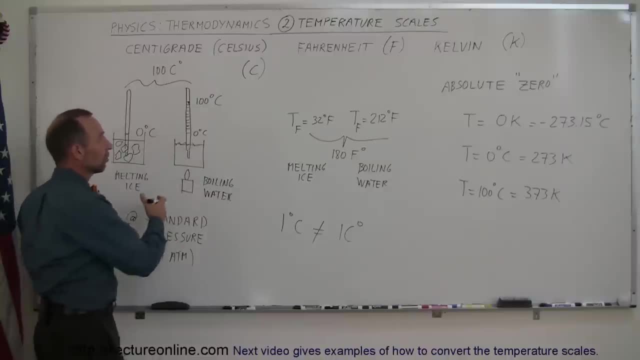 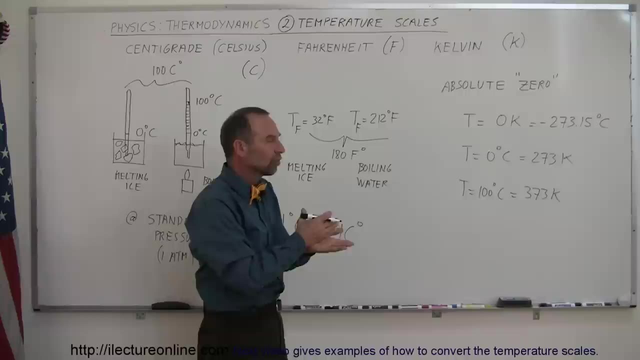 scales, how the centigrade scale was derived, To see how that relates to the Fahrenheit scale. and then, of course, we have the Kelvin scale. that is associated with the coldest it can ever be in the universe, which is minus 273 degrees centigrade.